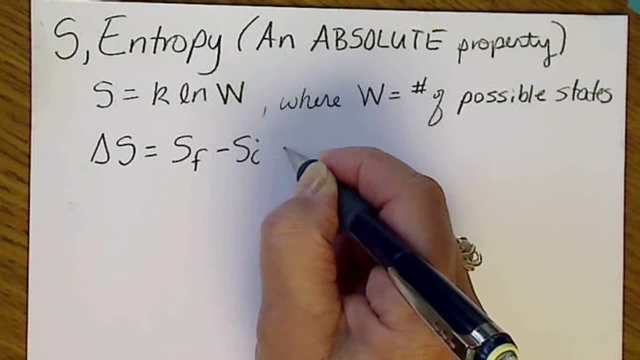 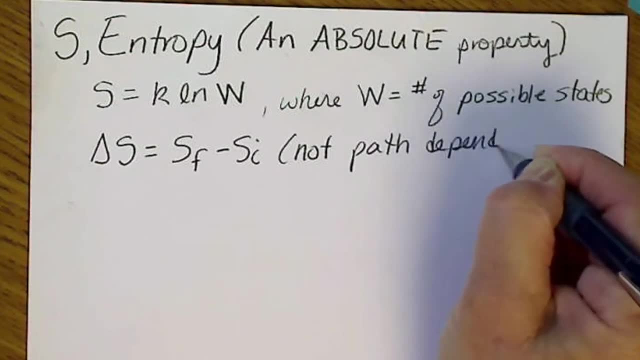 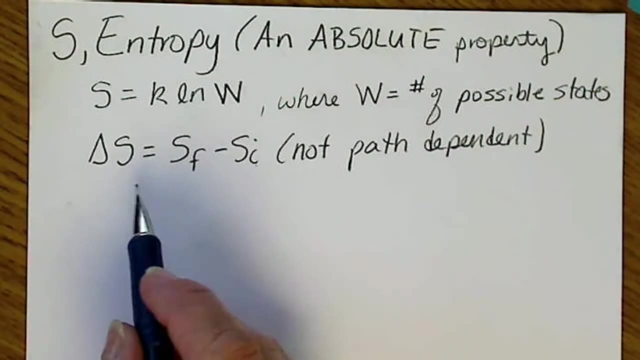 is S final minus S initial is not path dependent, So that means all we look for is the overall difference from the final state and the initial state. This definition of entropy S equals K times the natural log of W is the statistical definition and we are not going to use this. 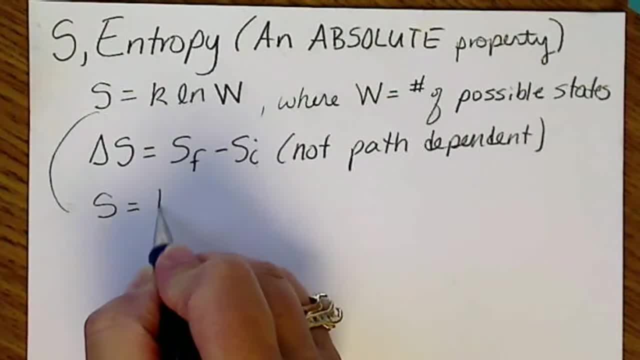 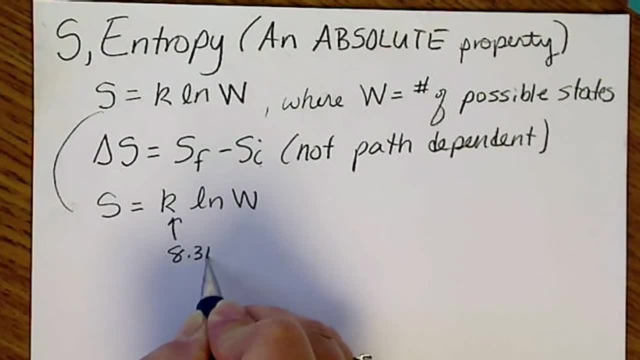 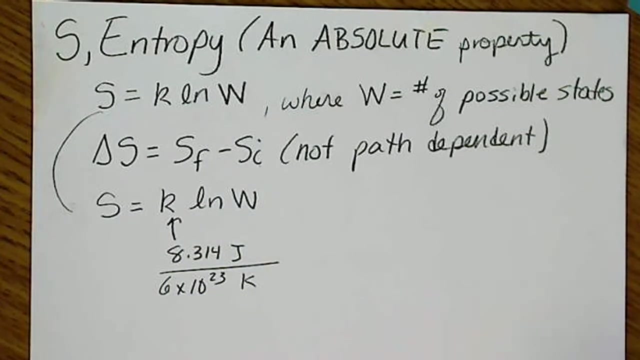 definition, But we'll take a quick look at it. K is Boltzmann's constant, So that is the universal gas constant in joules per mole, per degree kelvin. And when we divide by one mole then our mole cancels here. So Avogadro's number 6 times 10 to the 23rd basically takes the universal. 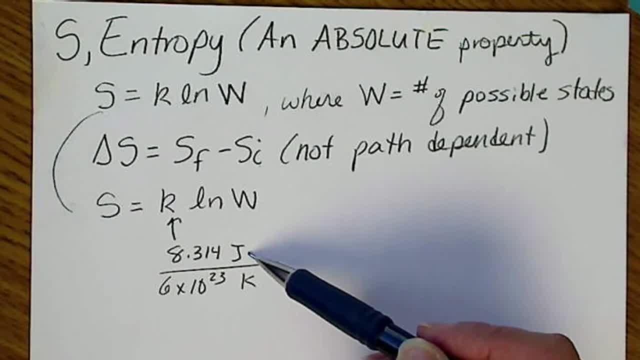 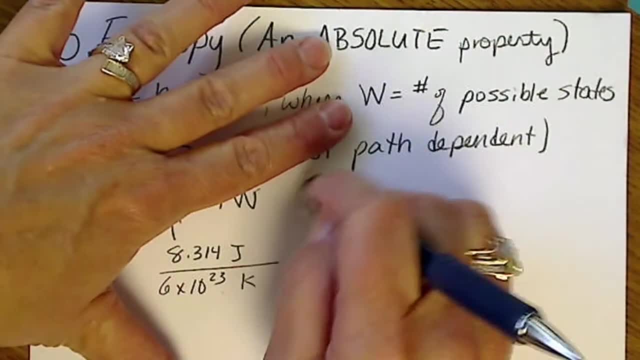 gas constant in terms of per mole in joules. So that's the universal gas constant in joules per mole and changes it into per item And W. well, I already wrote that here. W is the number of possible states, So from: 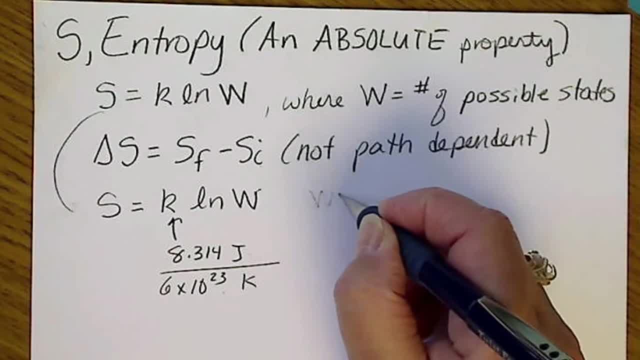 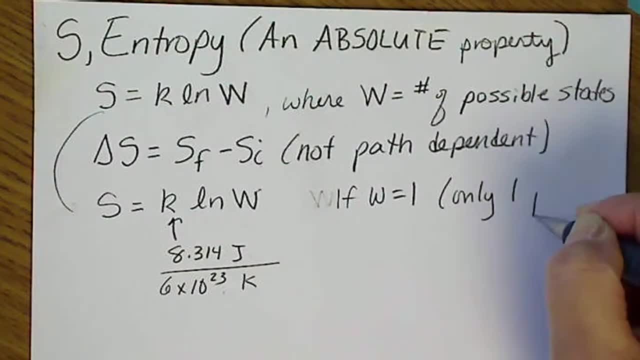 a statistical point of view, if W equals 1, that means there's only one possible state for a system to be in. And that's actually where we're going to be, Where we define the third law of thermodynamics, stating that at absolute zero degrees kelvin, 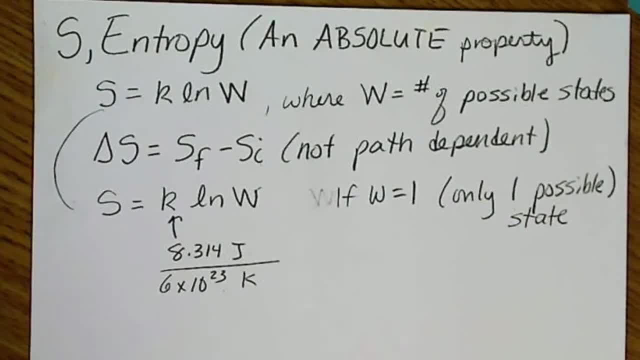 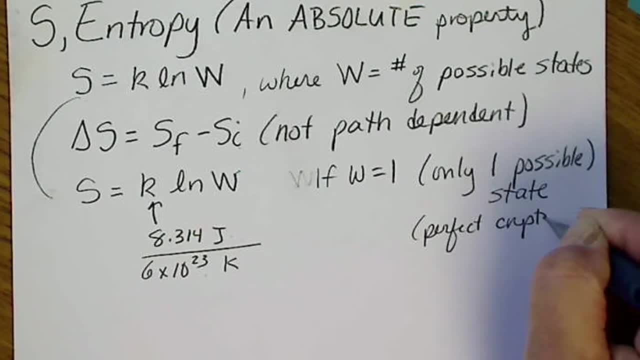 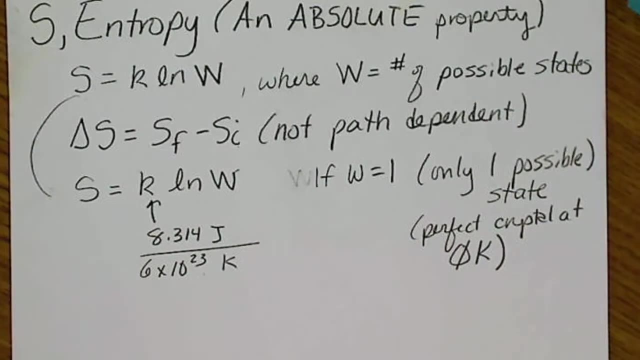 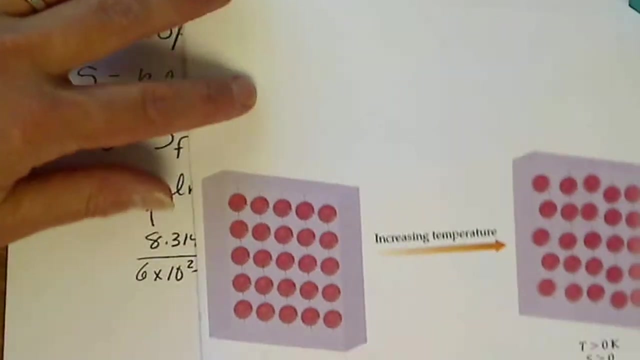 there is only one possible state for a perfect crystal to exist in, So I'm going to write that down here. So this would be a perfect crystal at absolute zero degrees kelvin- And I've got a picture to show us of that- And if we have a perfect crystal that has no defects in it, then it would be ordered. 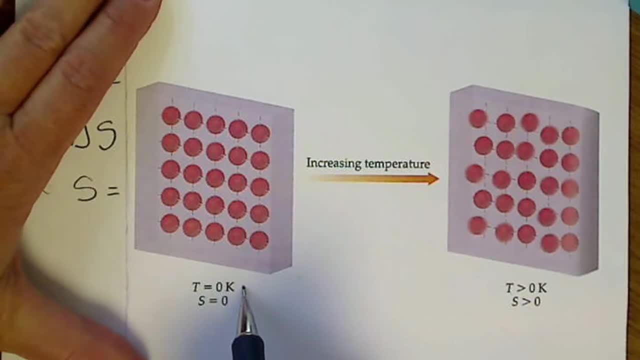 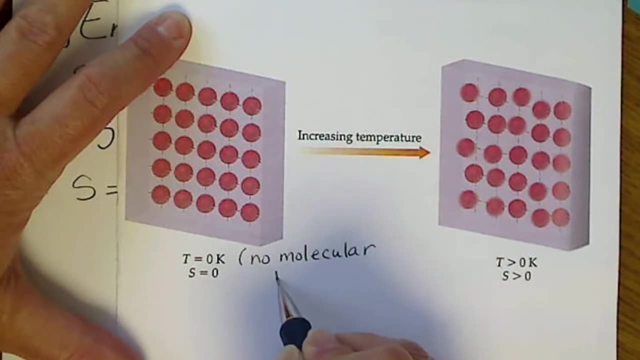 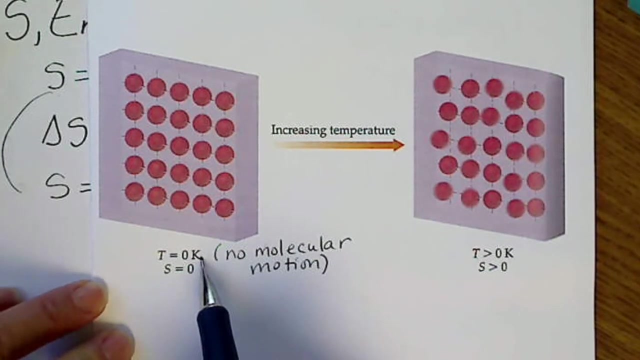 perfectly And at absolute zero degrees kelvin, there is no molecular motion. So remember, temperature is a measure of molecular motion. Temperature is not heat. Heat is a form of energy and temperature is a measure of energy, a measure of motion. So, if we can cool a perfect crystal down to absolute zero degrees Kelvin, 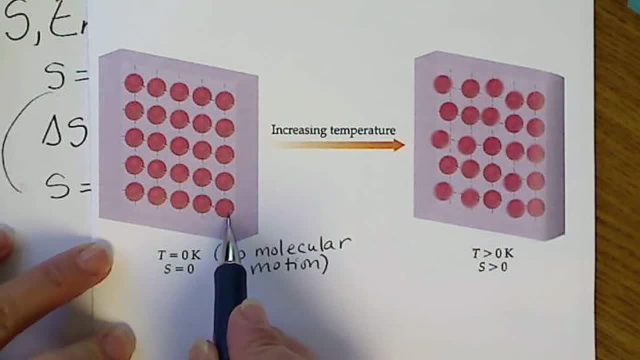 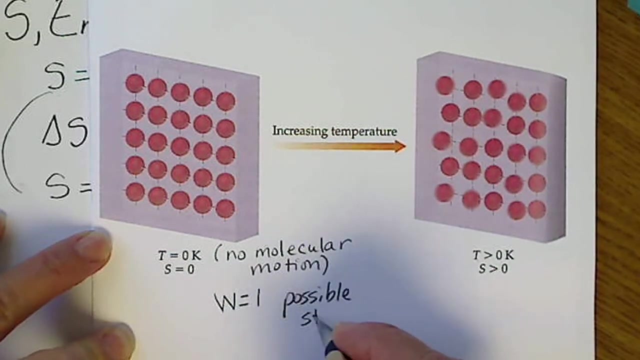 there's only one possible picture that we could see, And every time we look at this perfect crystal at absolute zero, it's going to look the same. So here W equals one And again, that's one possible state. So that's what W means. So if we look at the definition, 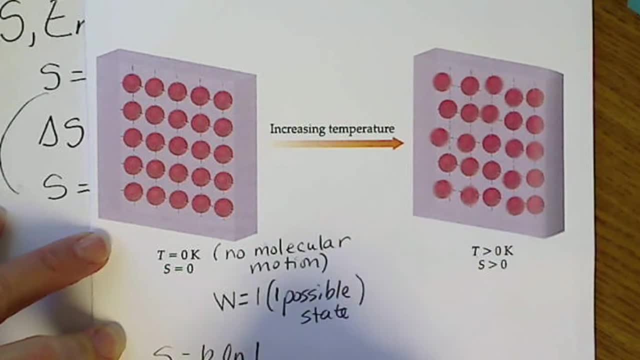 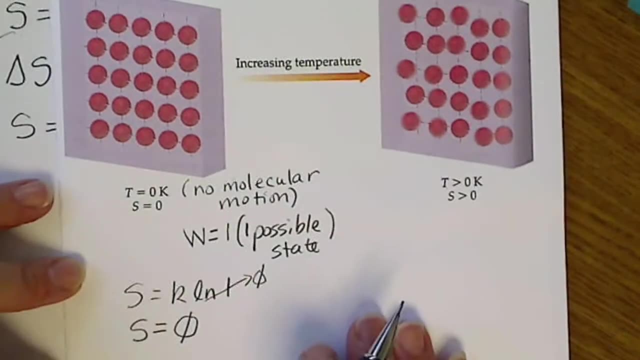 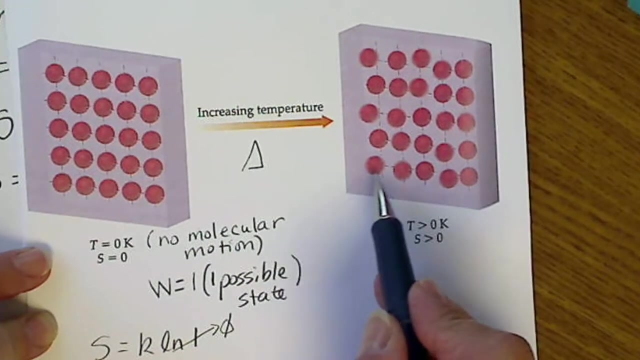 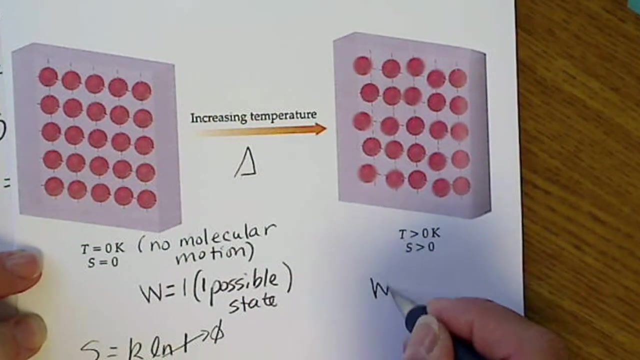 of entropy, the ln of one natural log of one goes to zero. So here we do have an entropy term equal to zero. As soon as we add heat to this, we start seeing motion, Motion from the atoms. So if W is definitely going to be greater than one here, So the 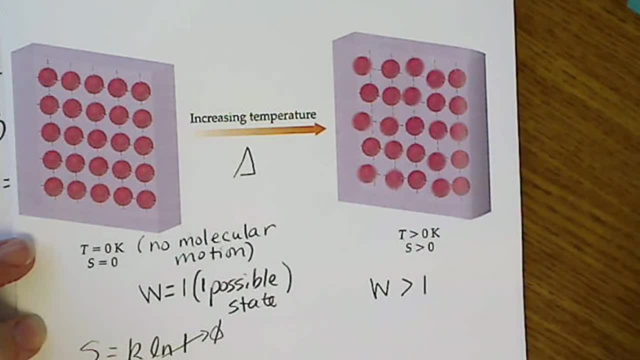 way we look at the number of possible outcomes. I think of it as though we're taking a photograph. We have a camera set up. We take a photograph every second, So if each photograph is not identical, then that means we have different states. So our third law of thermodynamics. 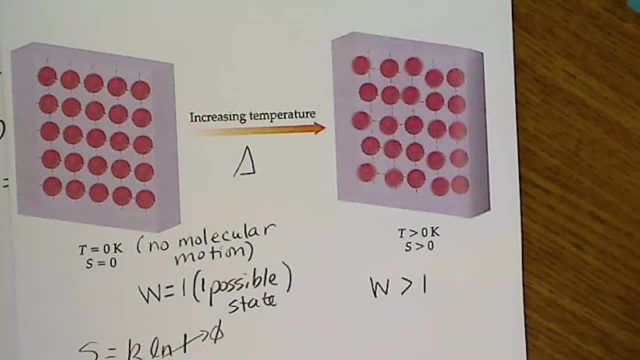 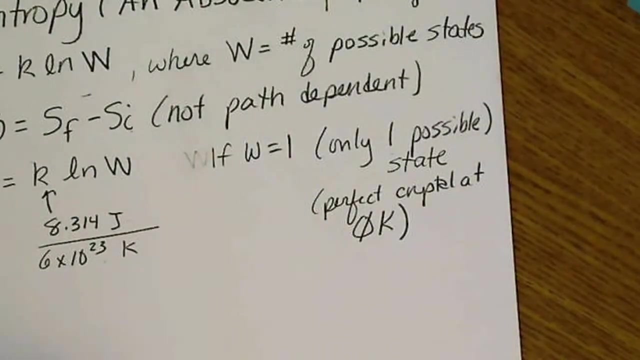 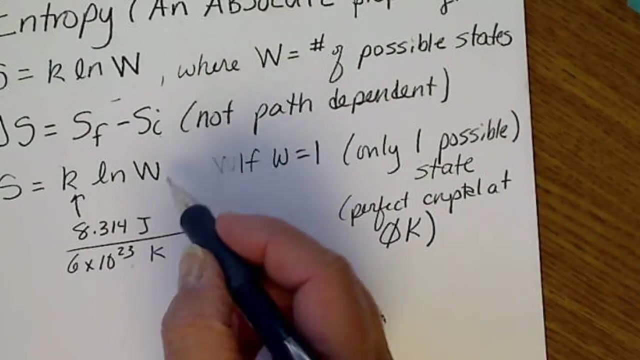 which defines Where entropy is zero. Wow, this is why this has to occur at absolute zero degrees Kelvin. So we're going to look at more of a qualitative view of entropy And we're going to care about the thermodynamic property. So we're really not going to use this. but from that picture, 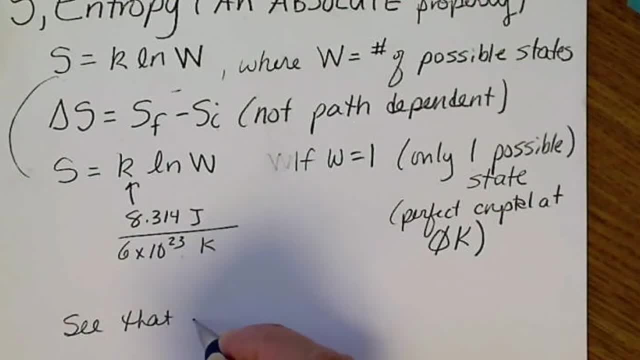 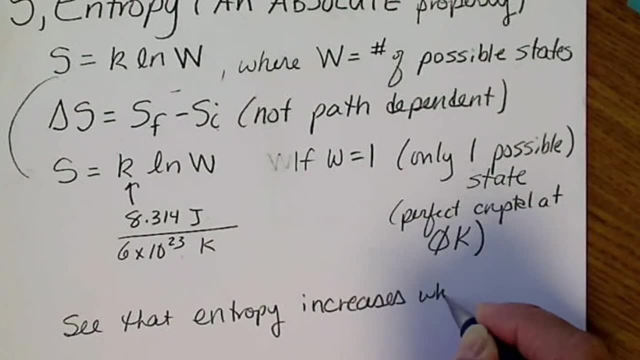 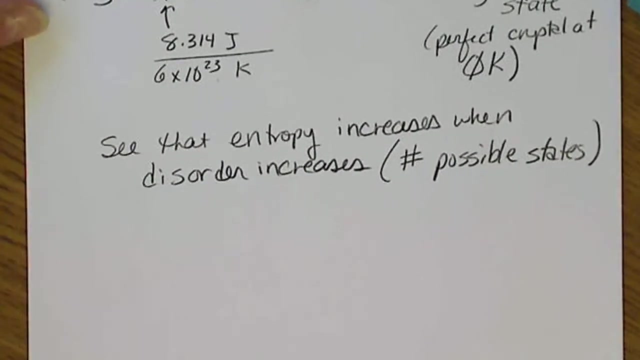 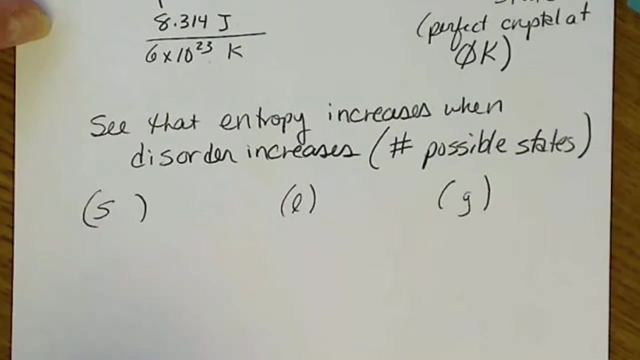 we can see that entropy increases when disorder increases, Or again, that's really the number of possible states that any system can be in. So for a phase change, if we look at a solid versus a liquid versus a gas, a solid is orderly. 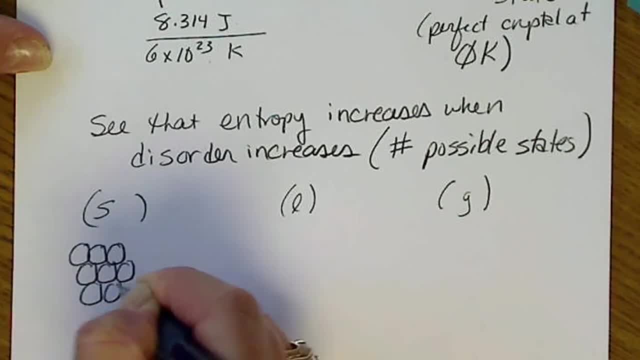 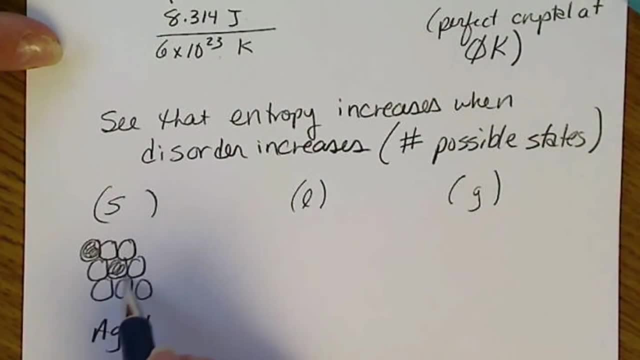 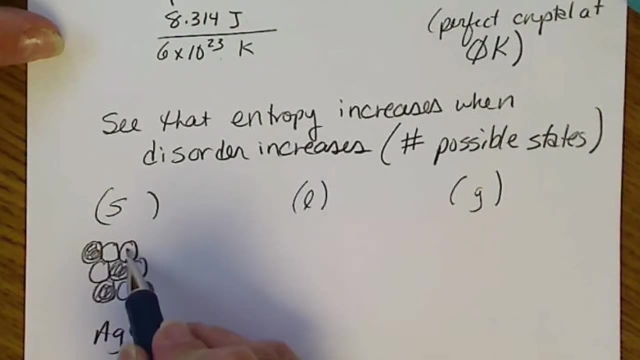 Maybe this is silver chloride. This might be a solid AgCl, which is a one-to-one ratio- a silver ion and a chloride ion, So we would have this one-to-one. If we heat this up, we'd have to get it to a fairly high temperature. 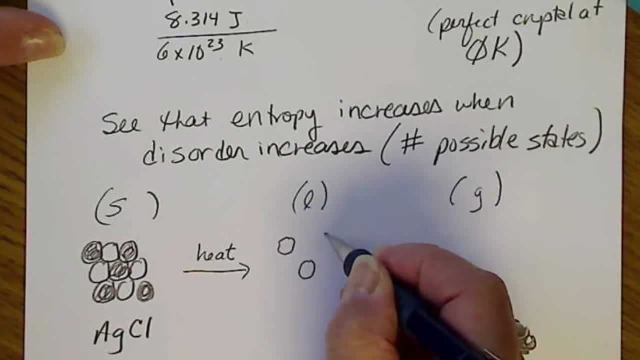 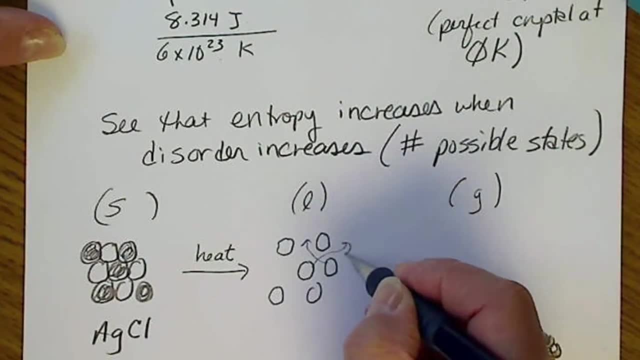 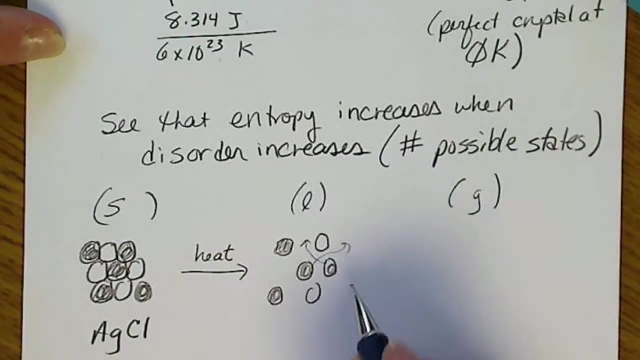 but we could get this in a liquid state or we could also get it in an aqueous state. So a liquid is less ordered and the particles are free to move with respect to each other. So melted silver chloride would have. 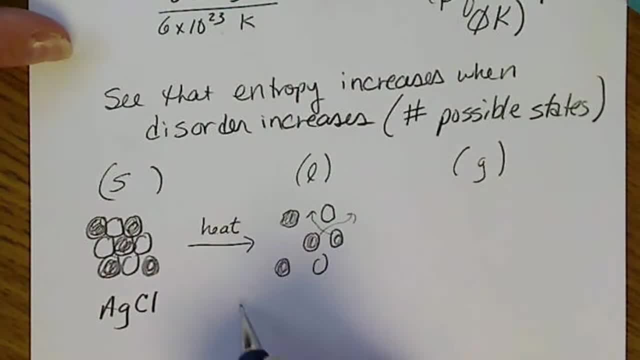 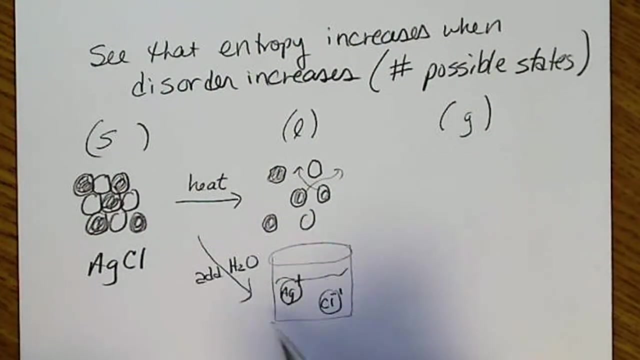 more disorder. or let's say we added it to water. That really makes more sense. Then we'd have aqueous silver chloride, in which case we'd have silver ions separated and dissolved in water. So melting a solid is very different than dissolving a solid. 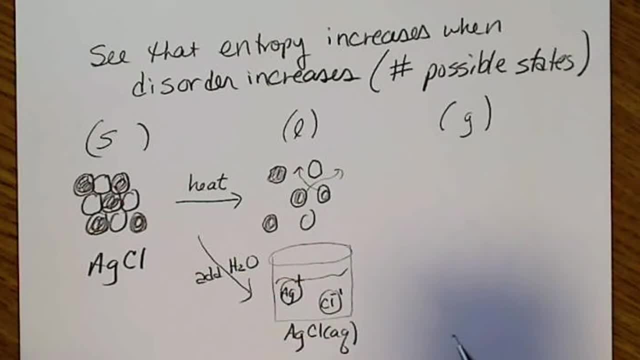 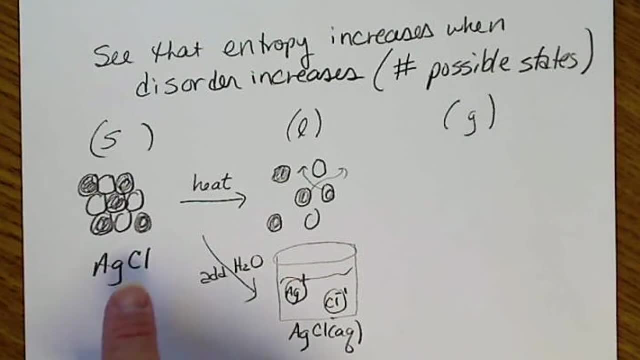 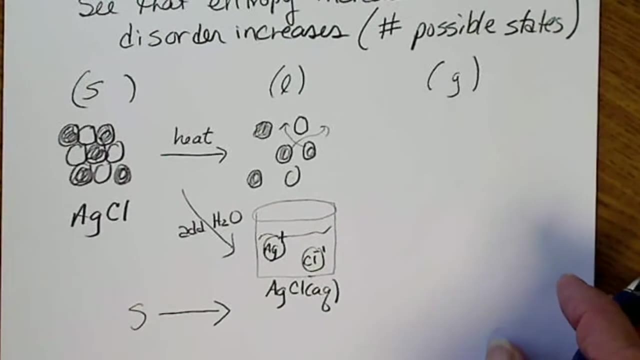 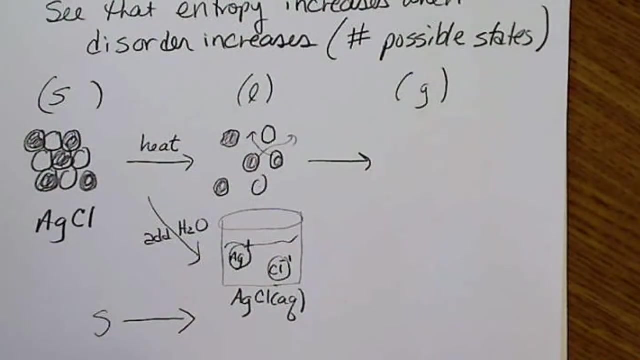 but in either case we would have more disorder in either of these states than the solid, So our entropy would be increasing in this direction. And finally, I suppose we could really heat silver chloride up to a very high temperature and turn it into individual atoms or a gas. 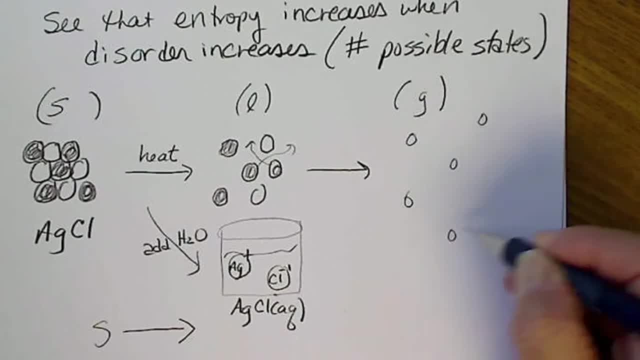 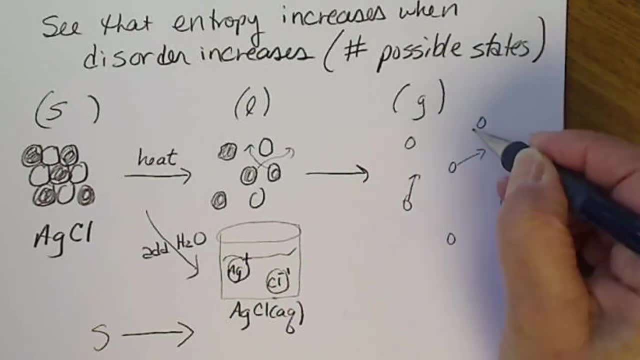 So I'm just going to drop any gas in general. So a gas, because it takes up so much space And each gas particle is in constant motion Every time we take a picture of the gas. if we could do that on a molecular level. 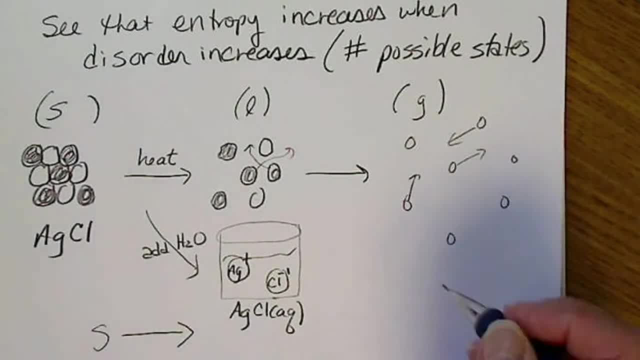 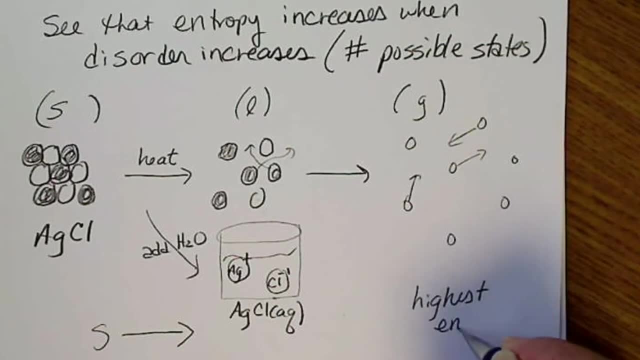 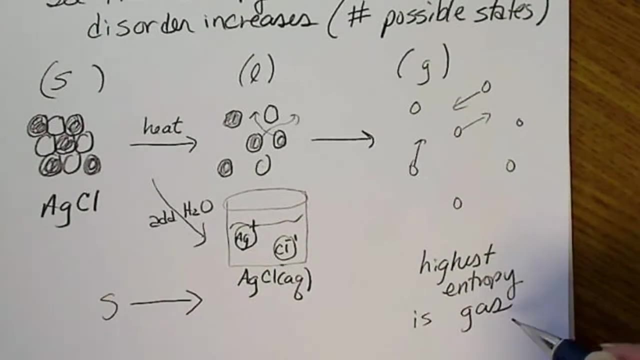 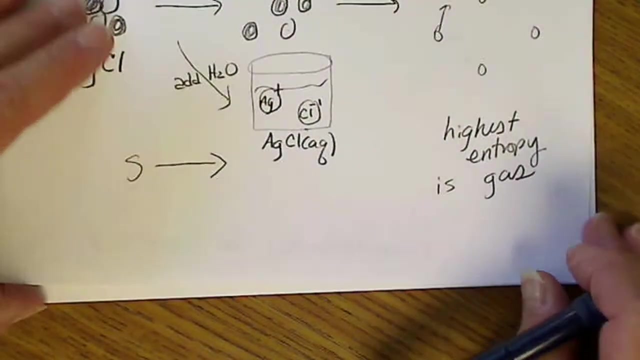 we would have a different photograph. So here: a gas is always going to have the highest entropy and a NOd, Alright, cool. And the more gas there is, the more disorder there would be. And I'm going to just talk about that for just a minute- what the values have to do with it. 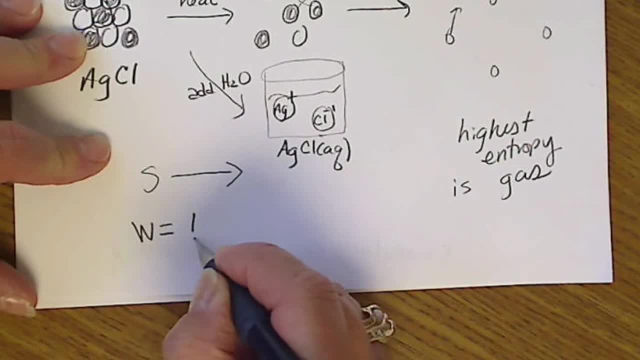 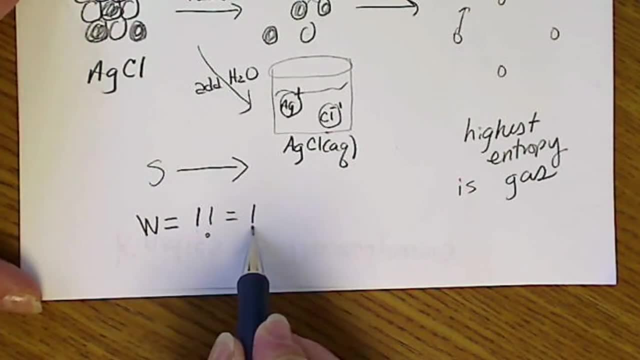 A lot of times the number of states is how many things you have, So one factorial equals one If you have one item. there's only one way for that to be arranged. If we have two items, two factorial is two times one, so we get two. 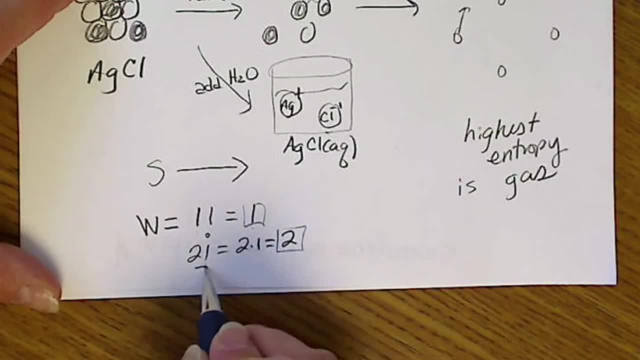 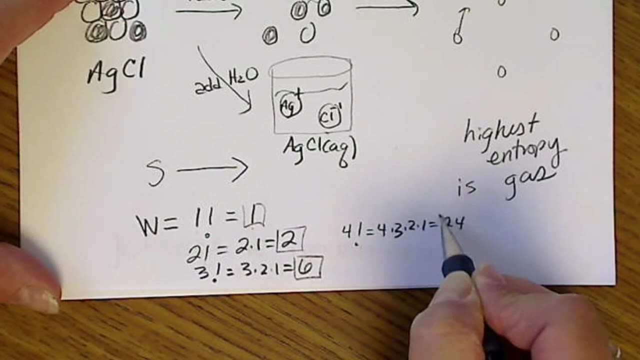 So two possible outcomes as opposed to one. Three factorial is three times two times one, which is six, And four factorial four times three times two, oops times one is 24.. So we can see from statistics that the The more items there are to rearrange, the much greater possible arrangements there are. 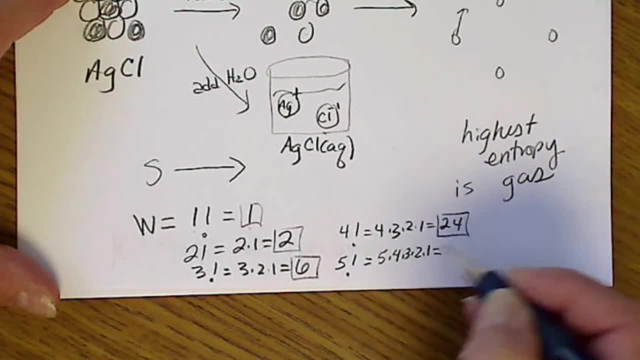 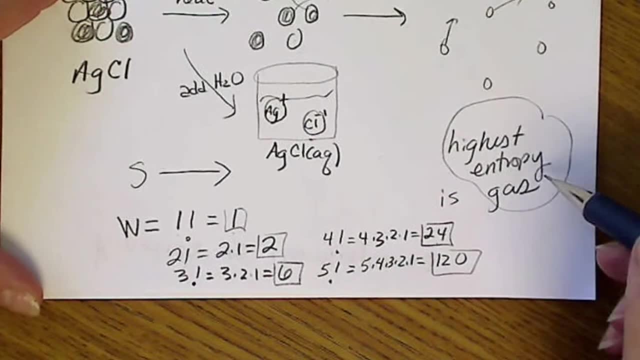 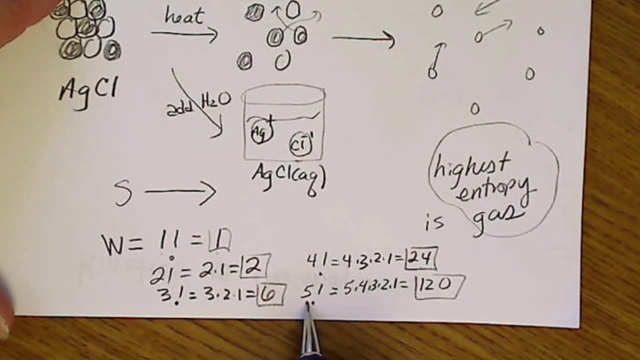 So five times, four times, three times, two times one is 120.. So the highest entropy is always going to occur for a gas, And also the more gas particles there are, or the number of moles of the gas, is going to increase the number of possible. 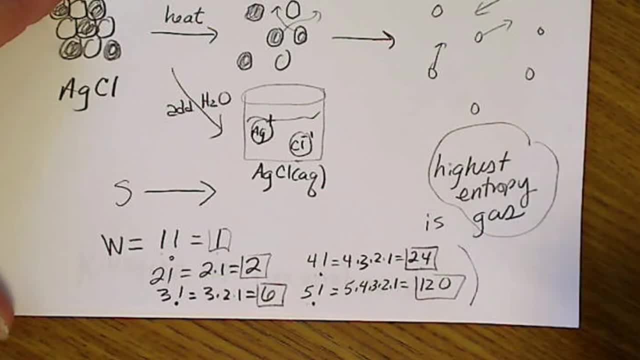 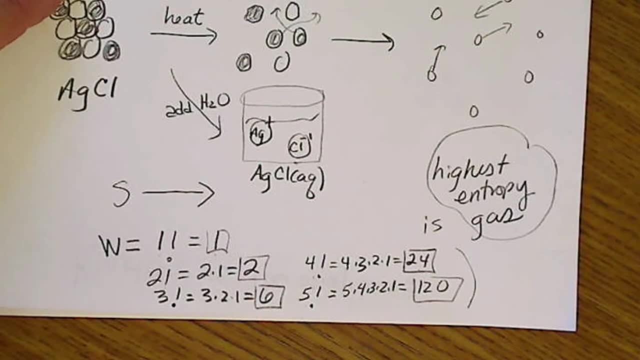 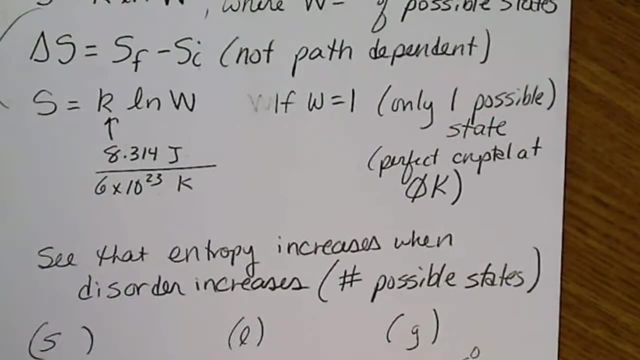 And this isn't direct correspondence here, but we're going to take a look at Just looking at any chemical reaction and seeing if the entropy change is positive or negative. And what we want to remember about entropy is we define entropy in terms of disorder. 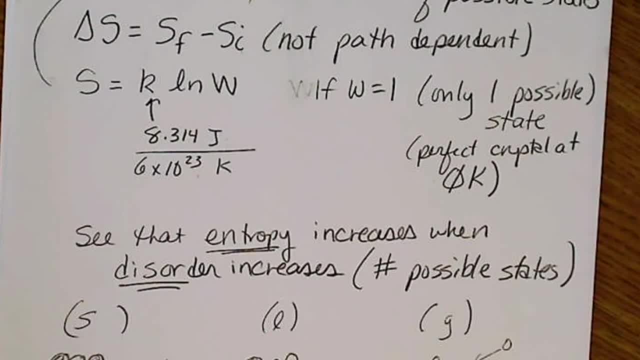 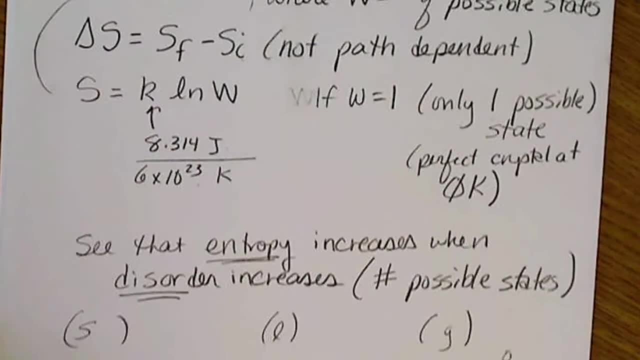 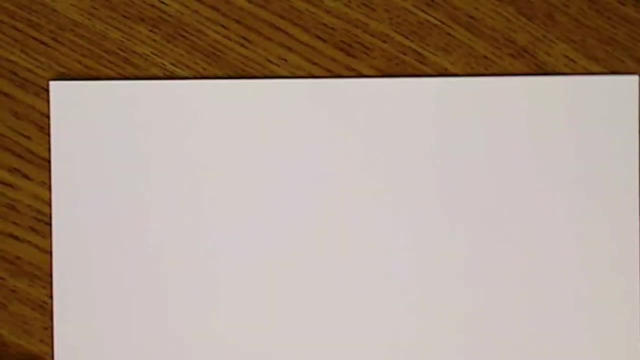 So usually we talk about how much something has, For example, How much order something has, not how much disorder something has. So we want to remember that with entropy, It's always a measure of disorder. Okay, So if we look, If we just think about this, 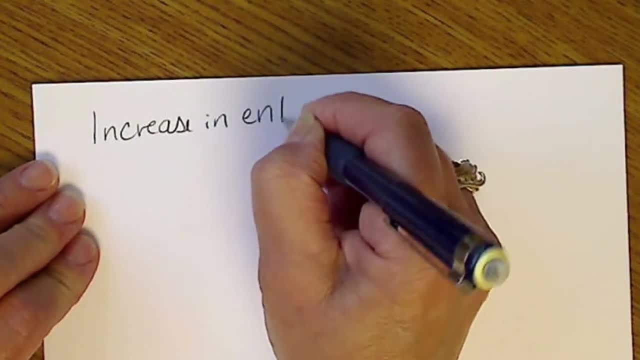 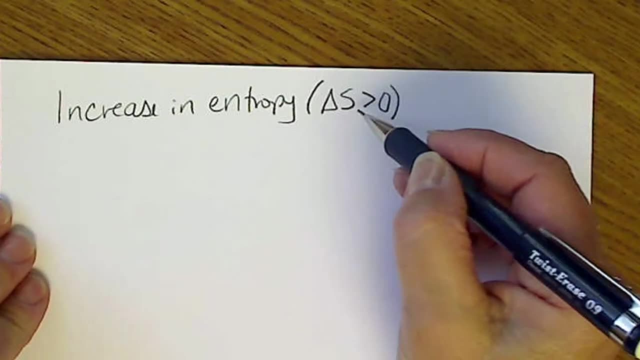 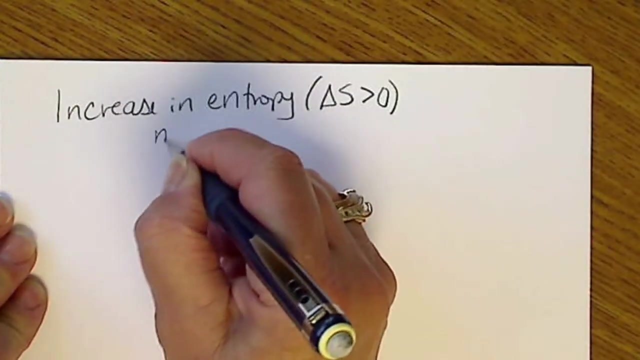 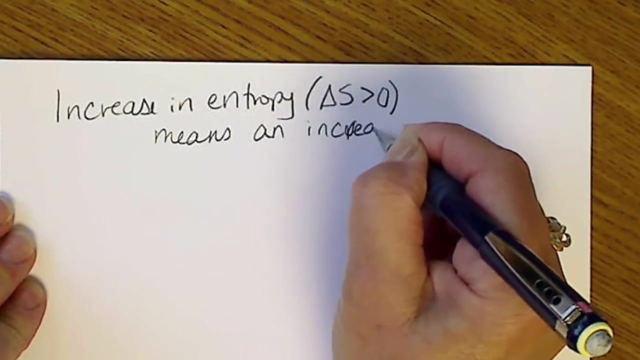 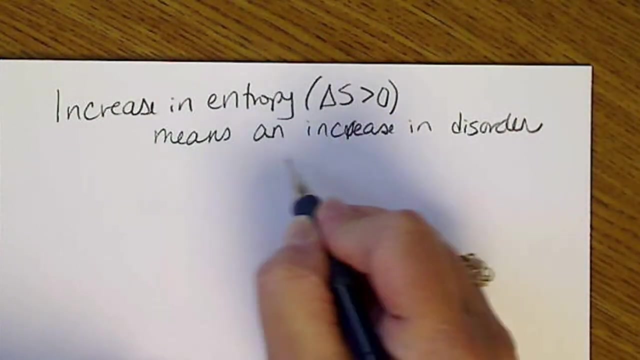 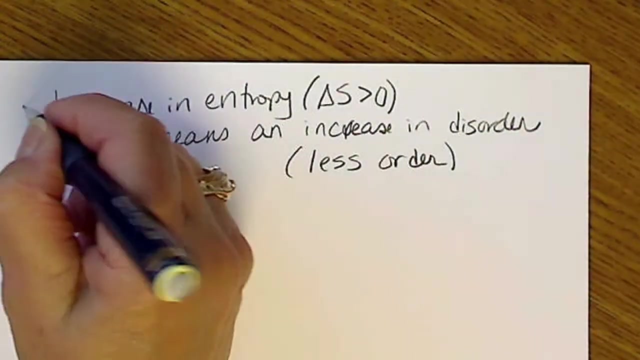 an increase in entropy. or we could write: delta: S would be positive, The final minus the initial would be a positive number. An increase in entropy means An increase in disorder. Or we could also think of that as less order And a decrease in entropy. 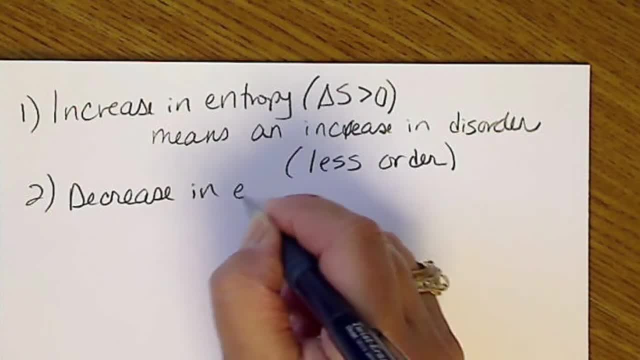 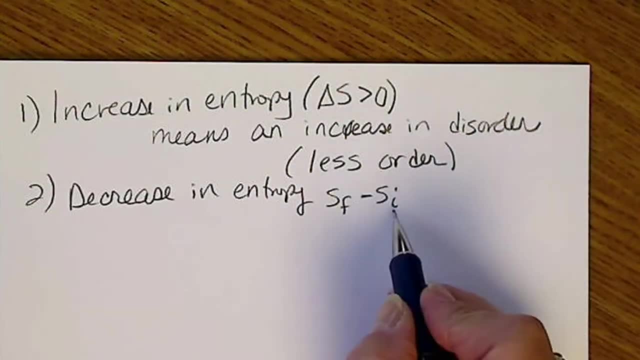 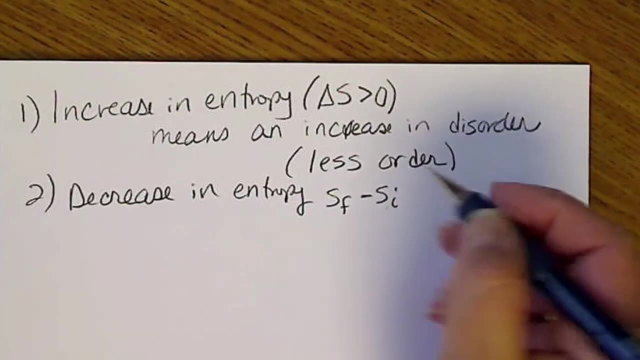 And a decrease in entropy. Or we could also think of that as less order. That means S final minus S initial. this is going to be a larger number. so we take a small number and subtract a larger number from it. that means our delta S is going to. 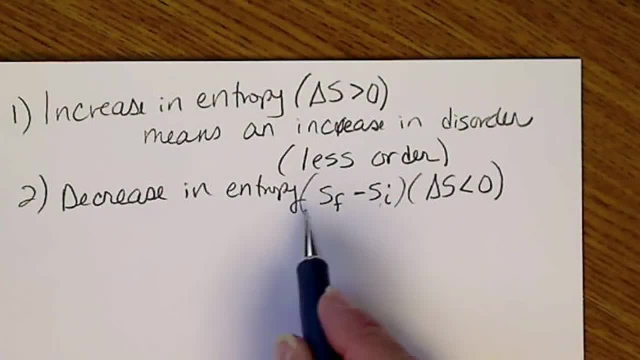 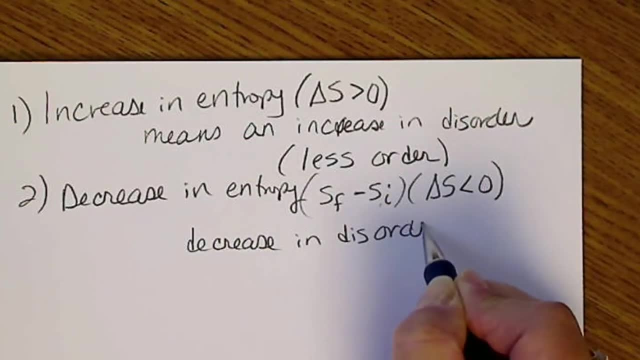 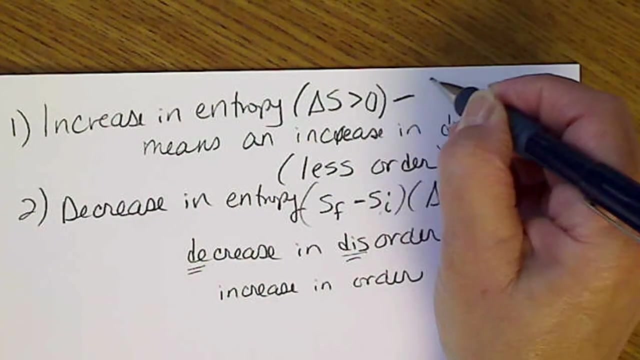 be a negative number. So a decrease in entropy is a decrease in disorder. So in a way this is like a double negative. we decrease disorder, so that's the same as increase. in order, This is the most favorable and we don't really have to go far to see that. if you look at. 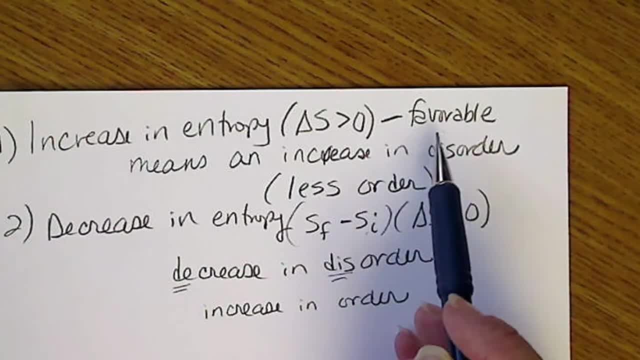 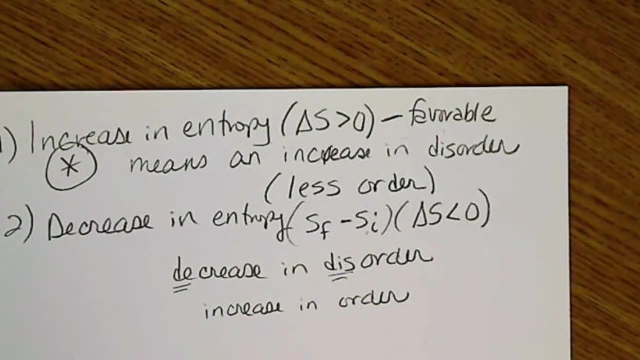 the top of my desk or you look at your shop door, it's apparent that the universe proceeds in the direction of going from order toward disorder. So this is going to be one of the criteria we look at when we decide or calculate whether a reaction is spontaneous or not. 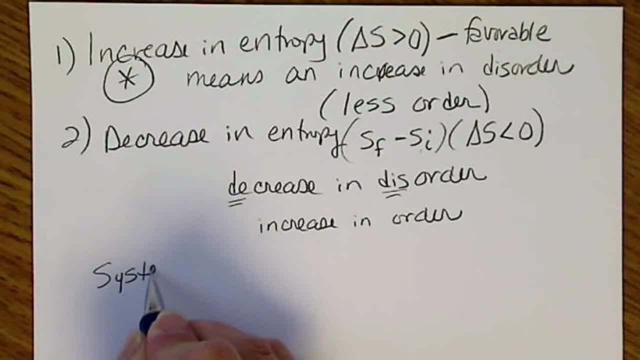 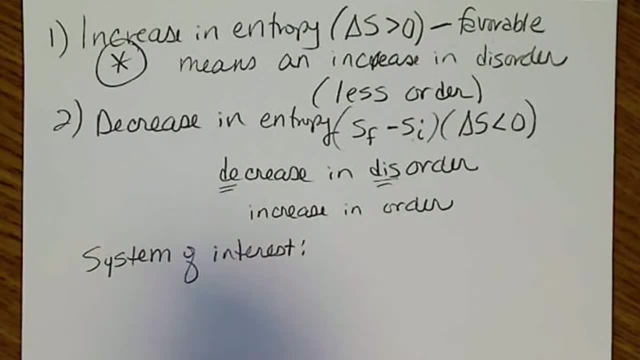 So if we look at a chemical reaction, for example our system of interest in chemistry, there's always going to be a reaction. and there is a famous reaction called the Haber process, which takes hydrogen gas and reacts it with nitrogen gas in the air, and this 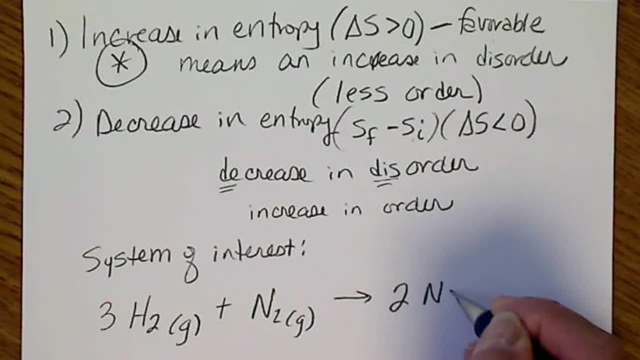 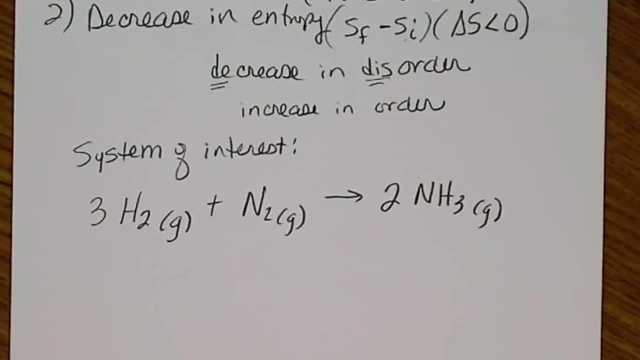 is a reversible reaction, but I'm going to write it: just going in one direction- making ammonia- And just from looking at the system, we can predict the system of interest, we can predict the reaction, we can predict the reaction and we can predict the reaction. so that's a lot easier. It's a lot easier to write down the whole system, Which, ever way you look at it, you will see that there's a lot of different reactions on different levels. So what we're going to do here, as well, is we're going to let the sender to do a little experiment here with these different reactions. So what you do is you're going to put these different reactions on the surface and you're going to ask the product to pass through the air and then pass through it And in the end you're going to 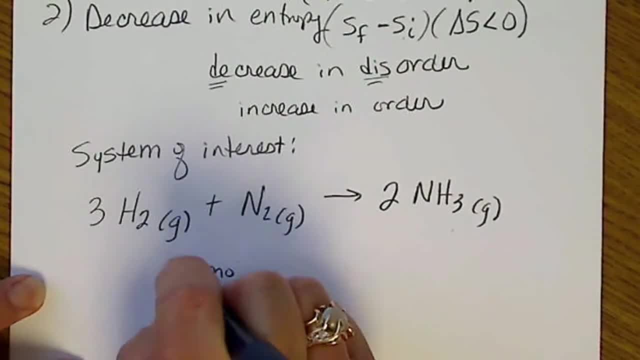 catch the reaction, And each time you do that, you are going to be able to get the reaction going. So this is a very effective example of a reaction, because it is a very good example of a reaction. So that is what we call a reaction. 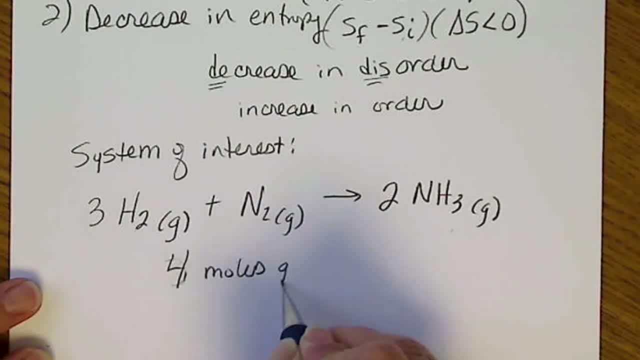 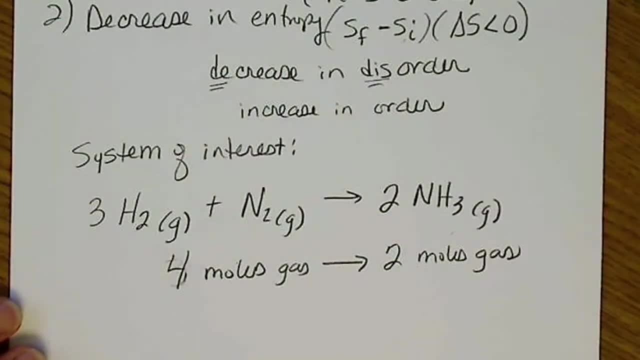 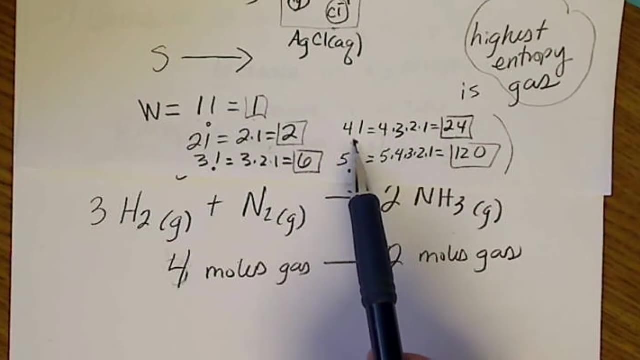 So this is a reaction. This is a reaction, moles of a gas reacting to form two moles of a gas And if we think about that number of possible states, four things can be rearranged many more ways than two things can. 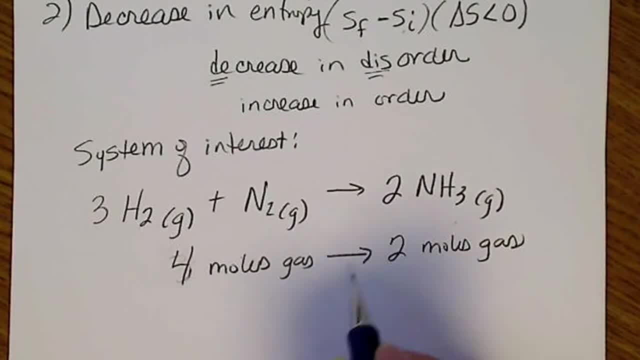 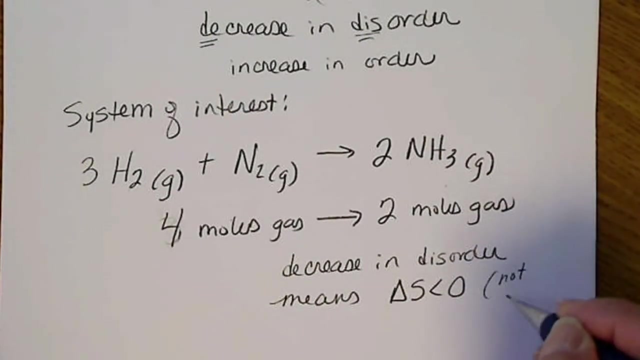 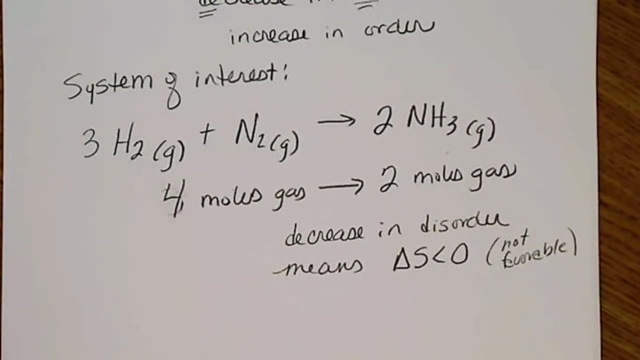 So, just from a statistical point of view, four gases going to two gases is a decrease in disorder. This means that the delta S term is negative or that it's less than zero, And this is not the favorable direction that the universe takes. We're going to take a look at this reaction in the next slide. 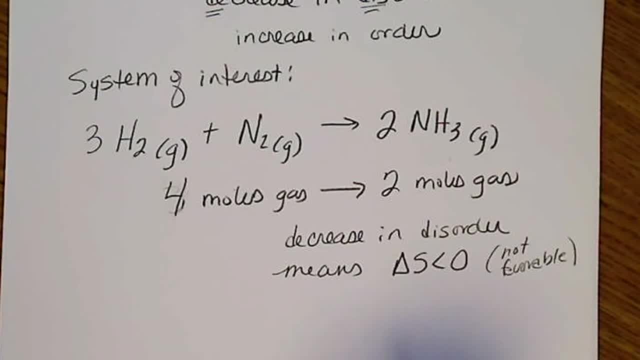 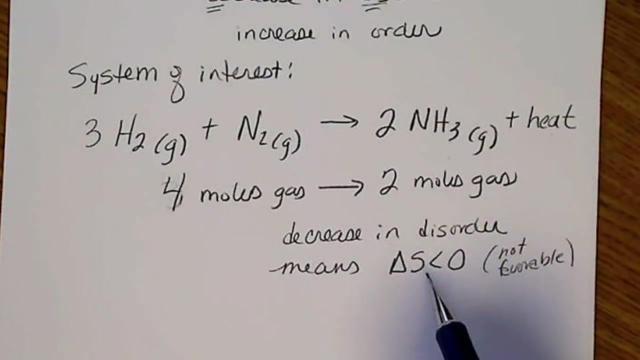 And we'll see that the other term, enthalpy, is great. So if we this reaction does proceed spontaneously, because it's an exothermic reaction And that term ends up in competition with the disorder term. So we're going to take a look at deciding whether a reaction is spontaneous. 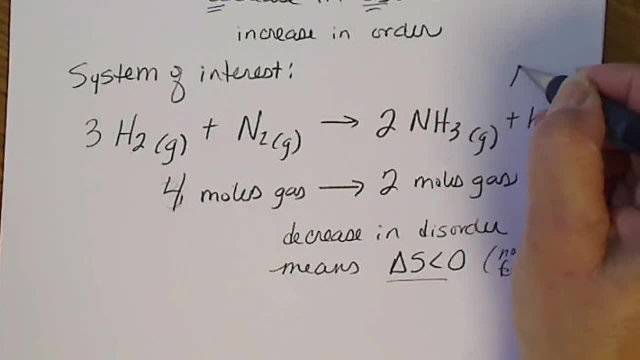 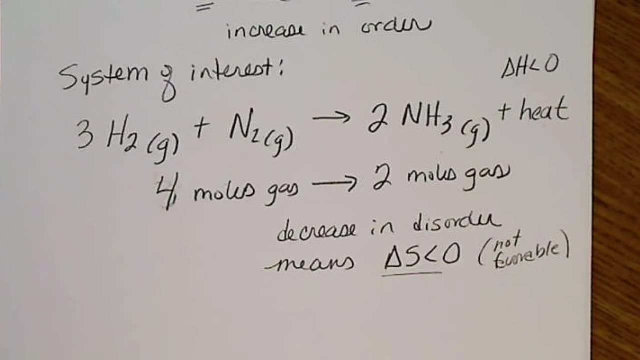 So we're not only going to have to look at delta S, but we will look at delta H. So that's coming up on the next slide. What we want to be able to do is just look at any reaction and decide whether the entropy is increasing or decreasing. 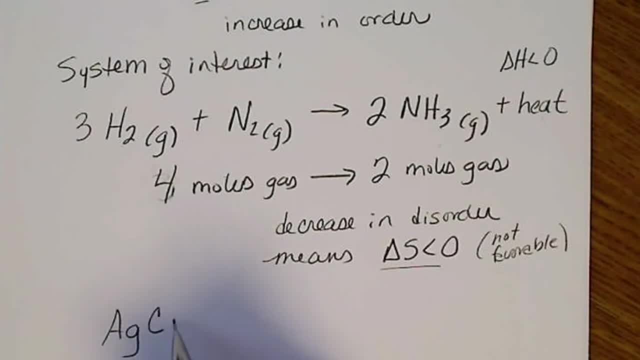 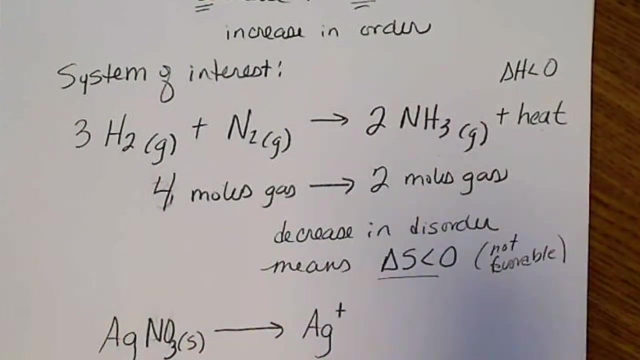 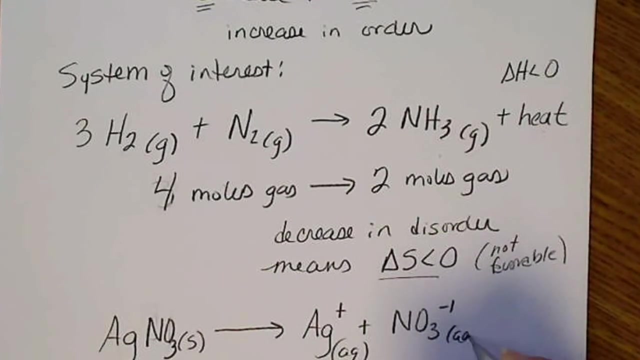 So if we have solid silver chloride and we dissolve that in water- actually that won't dissolve in water. we'll take sodium nitrate and we'll dissolve that in water. So the sodium nitrate will dissolve in water. So this would be our second example. 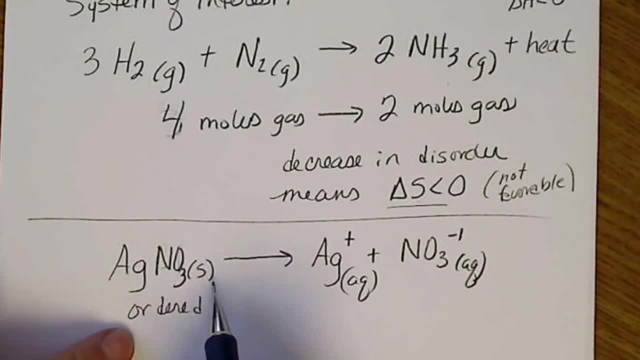 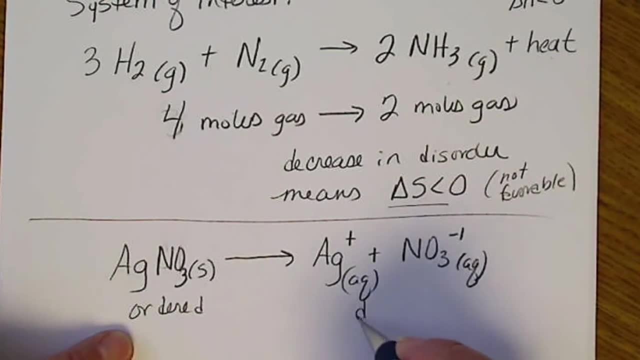 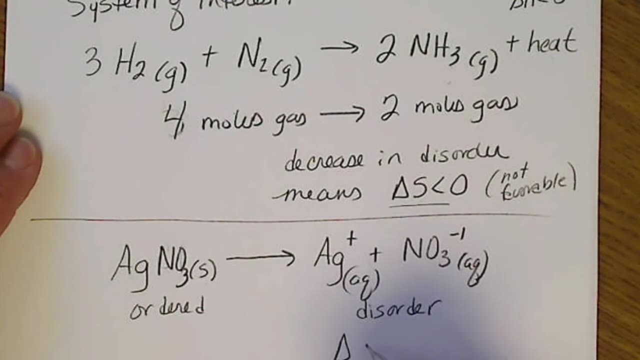 Here we have more order automatically because this is a solid, So we have an ordered arrangement in a lattice structure, And over here we have disorder because we have ions in solution. So we go from order to disorder. That means our entropy term is increasing.